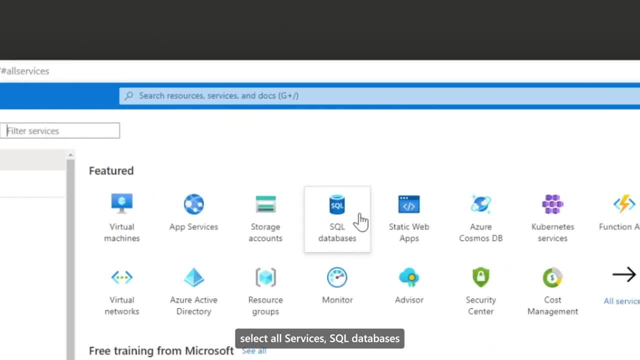 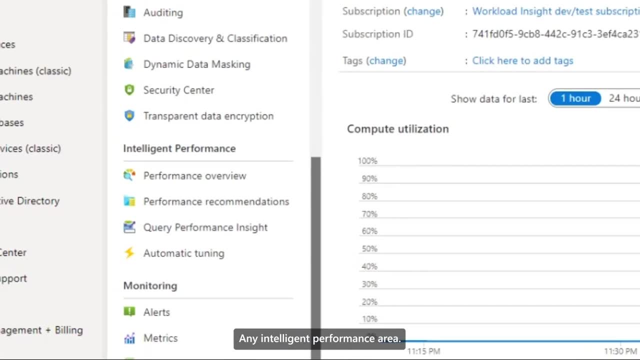 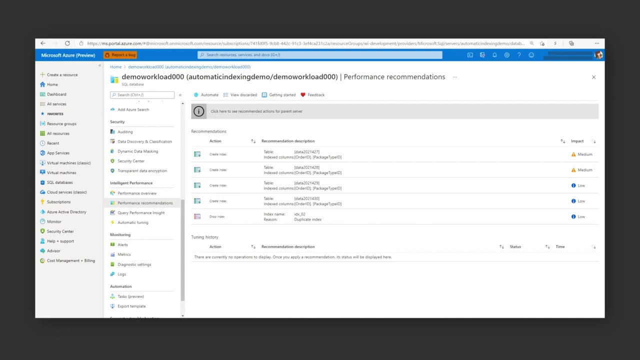 Azure portal: select all services SQL databases and then choose a database. In the intelligent performance area, select performance recommendations. If there are any, you'll see them listed as a table at the top of the page. The table displays the recommended actions in order of their performance. 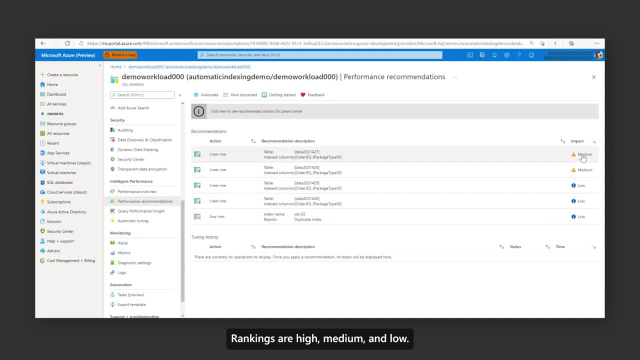 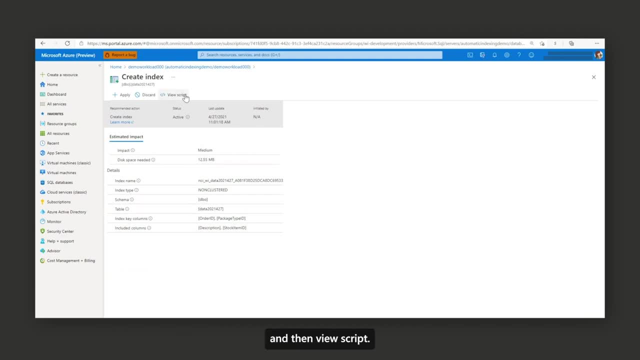 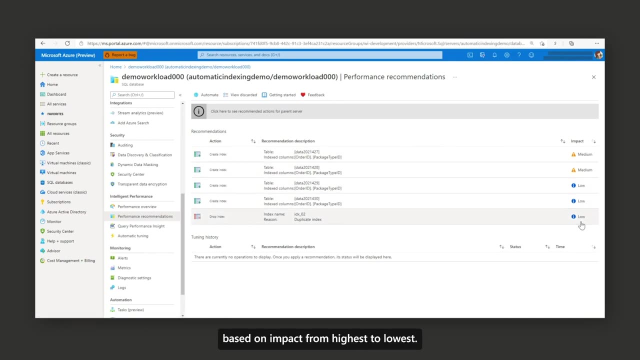 Theinese is the largest online application, with a range of more than 40 million services. You can see the details of each recommendation by selecting it and then view script. We recommend that you run each one individually, based on impact, from highest to lowest. After it runs, determine if there's any improvement. 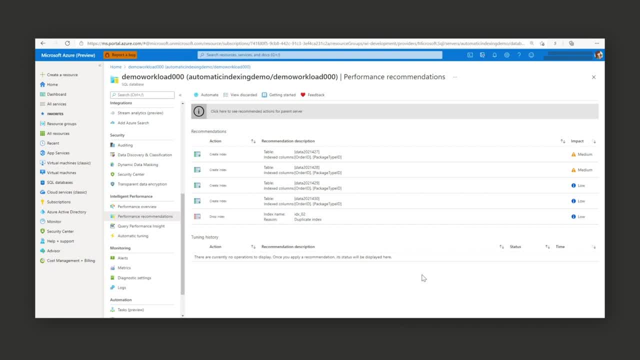 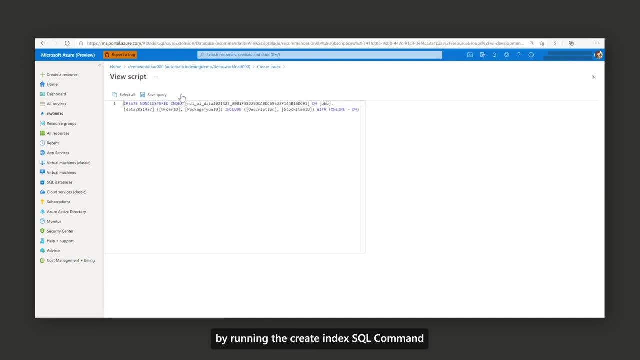 before you run the next one. If you have owner or SQL DB contributor permissions, you can run any of these recommended actions yourself. You can apply recommendations by running the Create Index SQL command or by selecting the Apply button. Running the SQL command allows you to immediately address the issue. 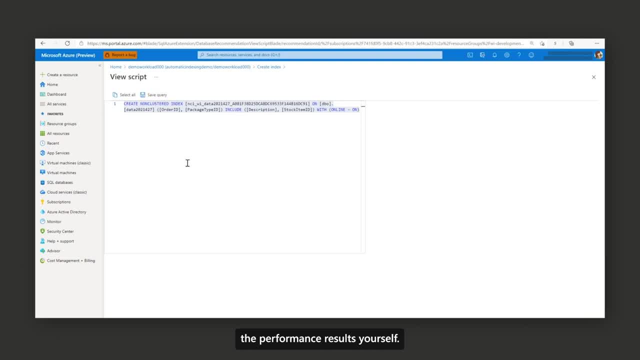 but it does require you to monitor the performance results yourself. The Apply button schedules the index creation when the database workload is at its lightest. However, this automatically verifies the index impact. To apply a recommendation, select one and on the Details page, select Apply. 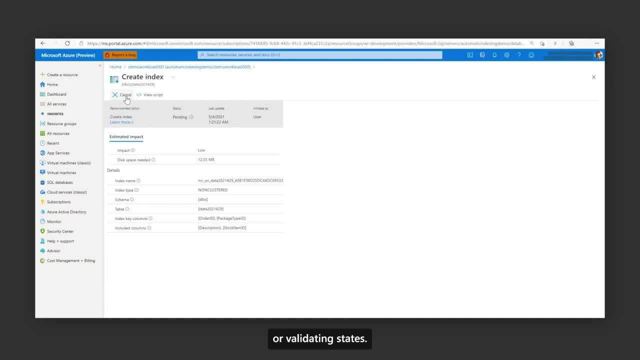 You can cancel a run when it's in the Pending or Validating states. If it's in the Executing state, it can't be canceled any longer. To monitor the performance results, you can run the Create Index SQL command or by selecting the 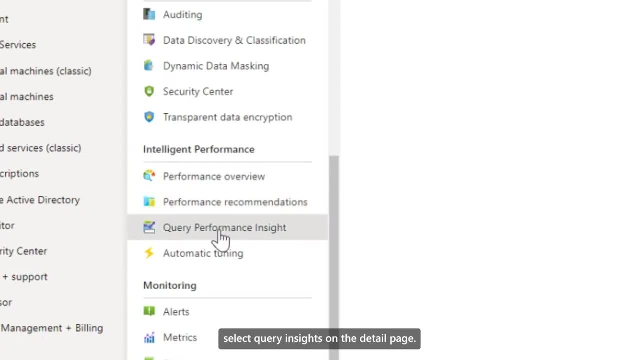 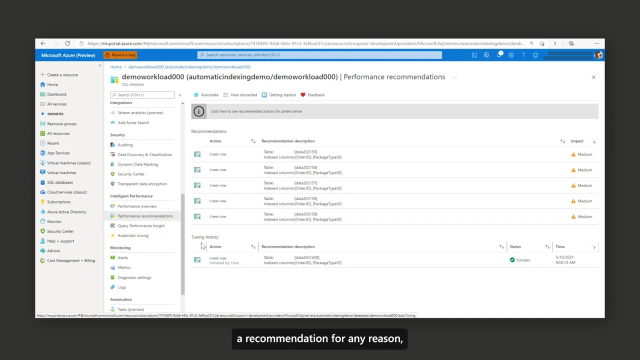 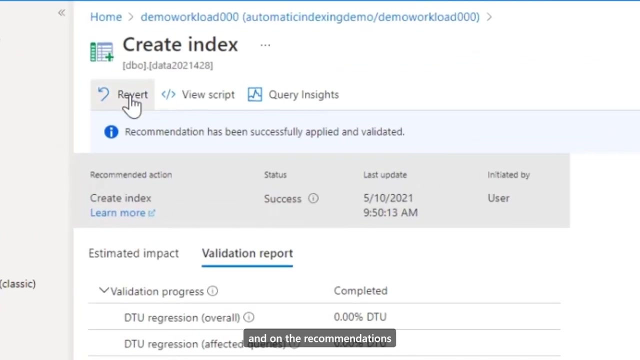 Apply button To monitor the performance impact. select Query Insights on the Detail page And if you decide that you don't want to keep a recommendation for any reason, you can revert it. Simply select the applied recommendation in the tuning history and on the Recommendations Details page, select Revert. Then it gets rolled back.